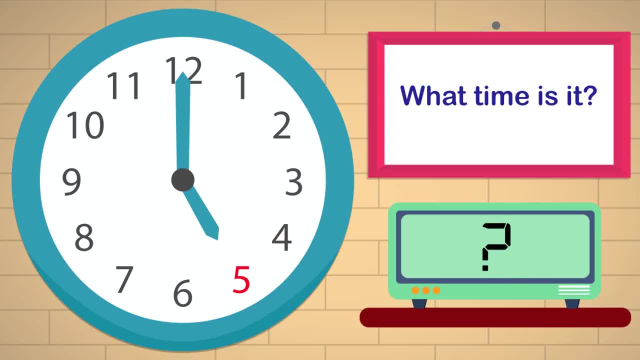 It's four o'clock. What time is it? It's five o'clock. What time is it? It's six o'clock. What time is it? It's seven o'clock. What time is it? It's eight o'clock. What time is it? 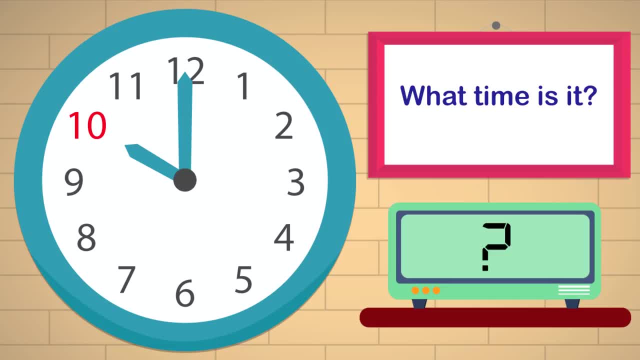 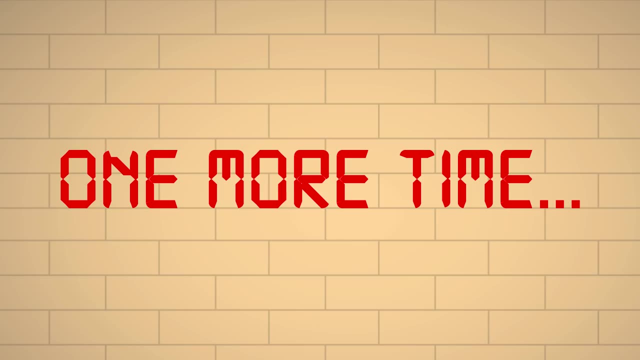 It's nine o'clock. What time is it? It's ten o'clock. What time is it? It's 11 o'clock. What time is it? It's 12 o'clock. Good job guys, Let's do it one more time. 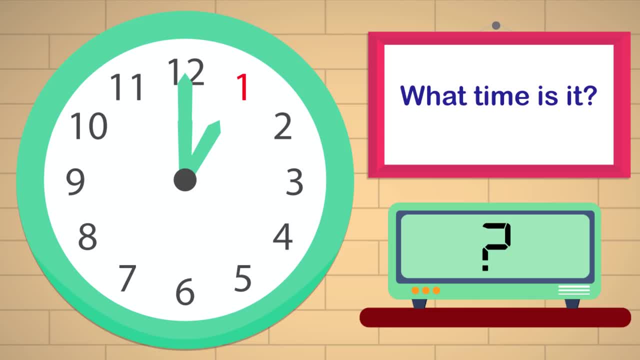 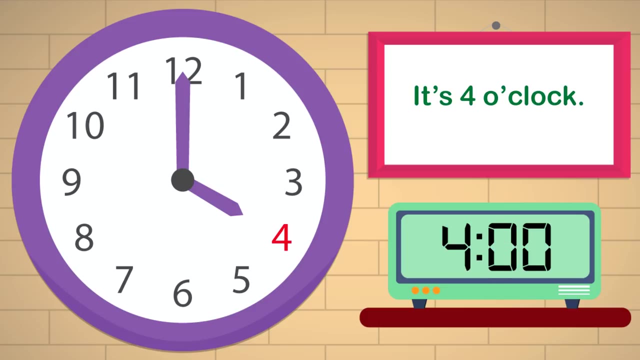 Ready, Here we go. What time is it? It's 1 o'clock. What time is it? It's 2 o'clock. What time is it? It's 3 o'clock. What time is it? It's 4 o'clock. 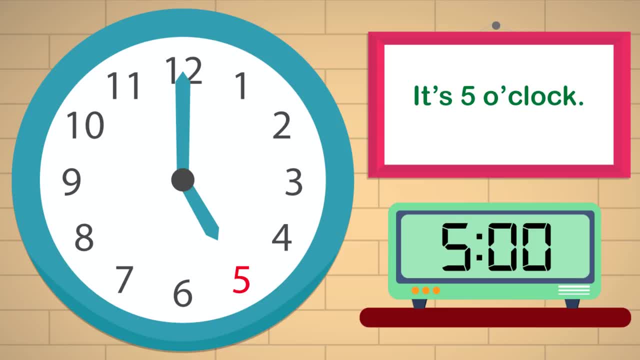 What time is it? It's 5 o'clock. What time is it? It's 6 o'clock. What time is it? It's 7 o'clock. What time is it? It's 8 o'clock. What time is it? 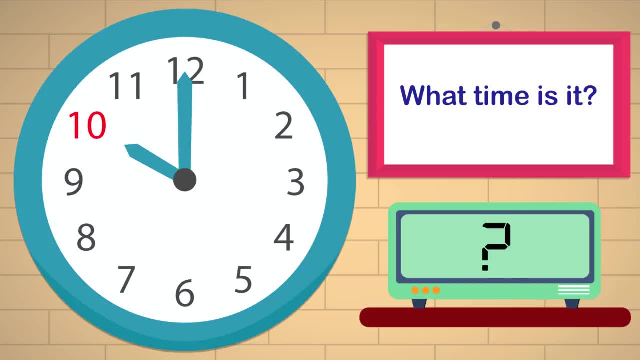 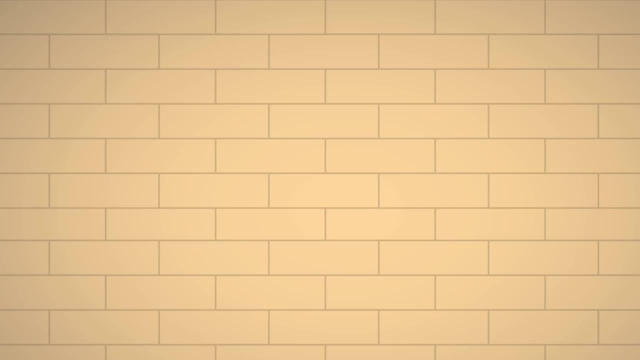 It's 9 o'clock. What time is it? It's 10 o'clock. What time is it? It's 11 o'clock. What time is it? It's 12 o'clock. Another great job, guys. One more time. 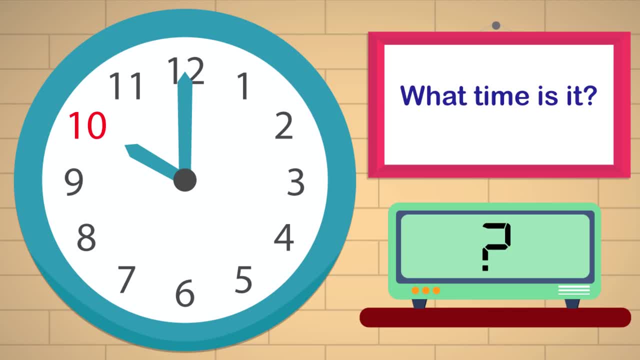 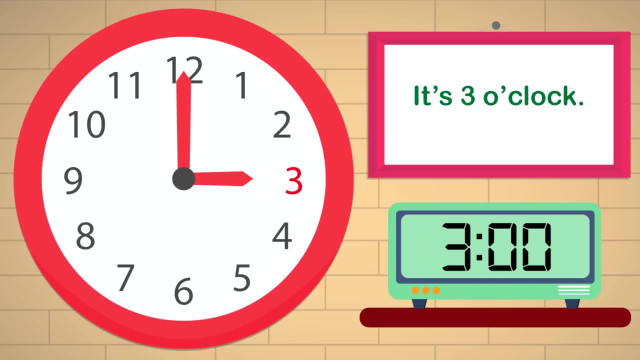 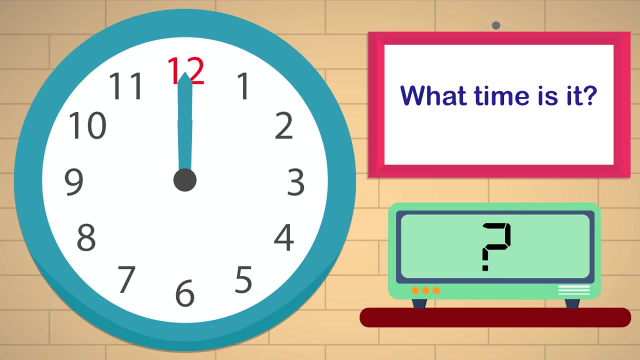